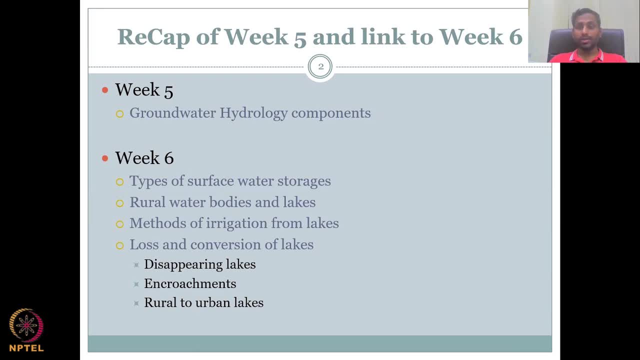 we then further progressed on finding the measurements and data where it can be available. We also looked at the role of groundwater in the water, The overall hydrology. Now, moving on, since we have looked at the groundwater as an important resource, we will 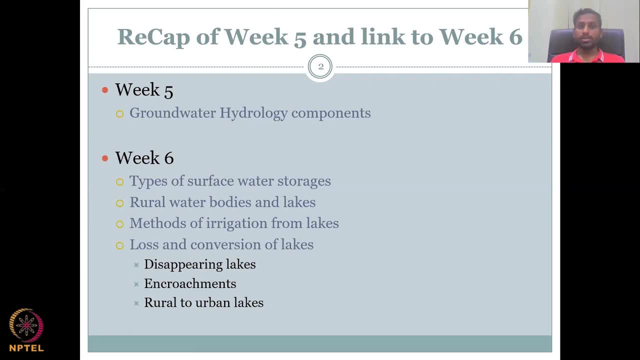 look at the other resource which is very important, which is the surface water hydrology. So in this week- week 6,, we will be looking at the types of surface water storages, mostly in the rural regions, because we are dealing with rural water resource in this course. 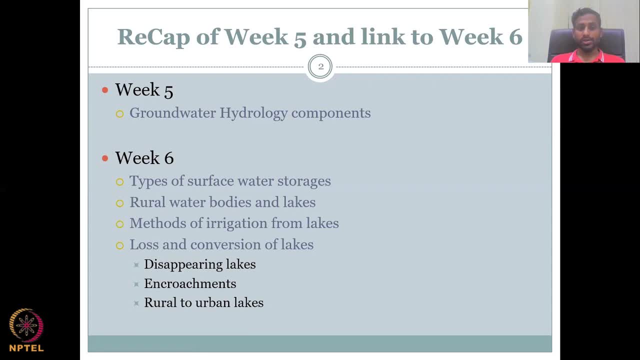 We will also look at rural water bodies and lakes. We will look at methods for irrigation from the lakes, For example. how do you take water from rivers and lakes within the rural system? It's not only a running water, but also stored water. 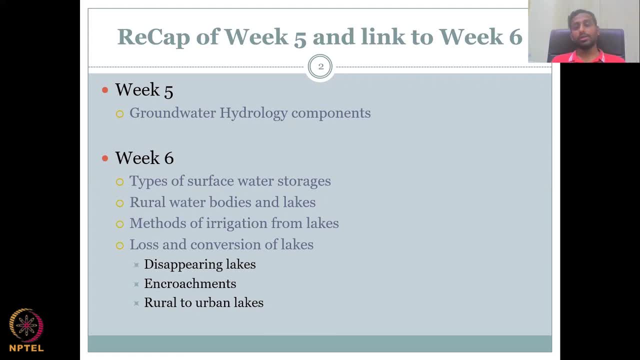 So ponds, lakes, etc. etc. And then there's a big concern on spots. Wait, what is a water supply system? So this is water storage. We have to look at what our water supply system is. what is being happening in the current scenario? most of the villages are experiencing loss and 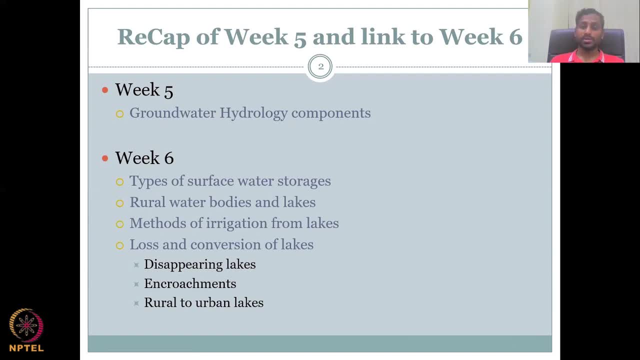 conversion of lakes. we will look into why this phenomena is happening, wherein we have disappearing of lakes, encroachments and conversion from rural to urban. disappearing is also kind of rural to urban, but most of the time disappearing just means that the entire lake or water body is drained and then construction is built on top of it. 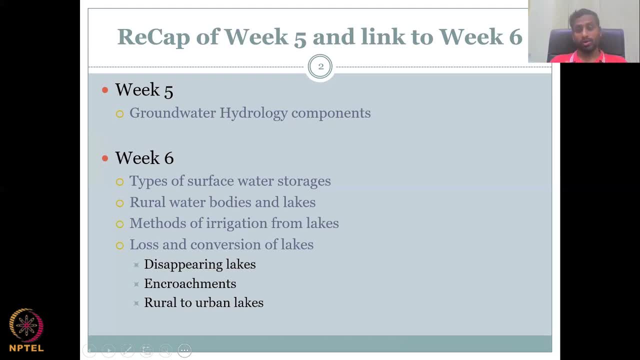 or, like in kerala, you have vegetation growing on it or agricultural crops. encroachments is where you block the water so that you drain it indirectly, and rural to urban conversions is again like where the urban center is increasing in size and some villages on the on the boundary of the lake are being drained and then construction is built on top of it. 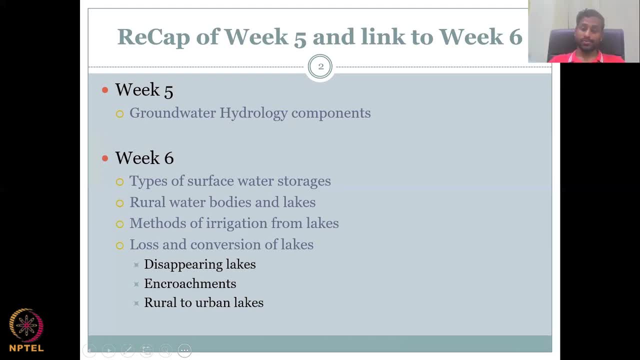 the urban setting are losing the water bodies. please understand that water bodies are government property and it has under no one's name, and so the boundaries are kind of very not stringent. there is no exact length, because one day the water body would be big and then one day, because of summer, it will be small. right, so there is a demarcation. however, 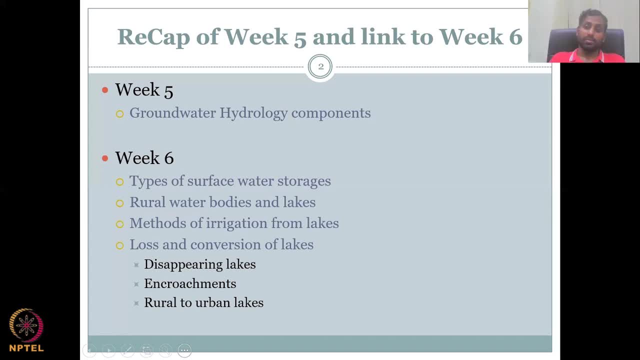 people don't know and they start to encroach it and abduct it, saying that that is their land. this is the key reason why in bangalore, we have a lot of lakes that are lost. so let's dive into week six. first, why do we need surface water storage? we talked about groundwater storage. yes, 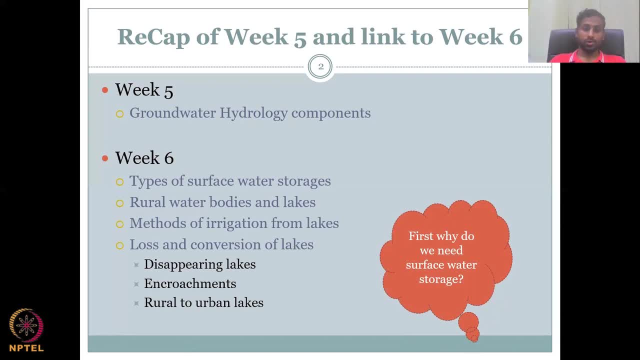 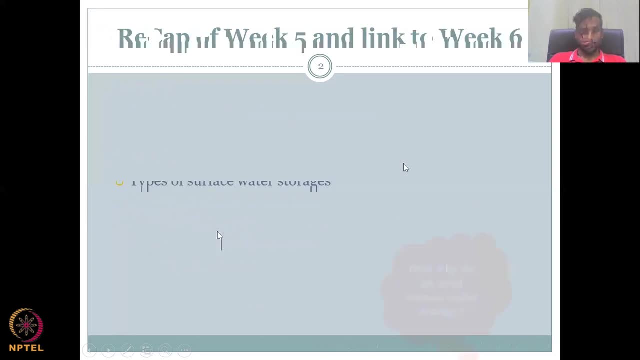 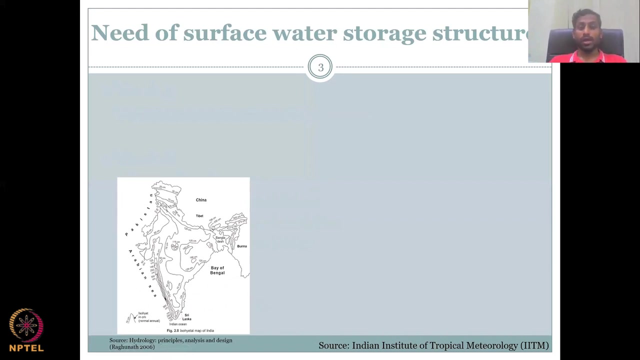 but there are specifics to why we need surface water storage. let's look into details. the need of surface water structures first. this image we saw in the early part of the course, wherein we have a variation in rainfall. if you look at it, the rainfall is not the same across. 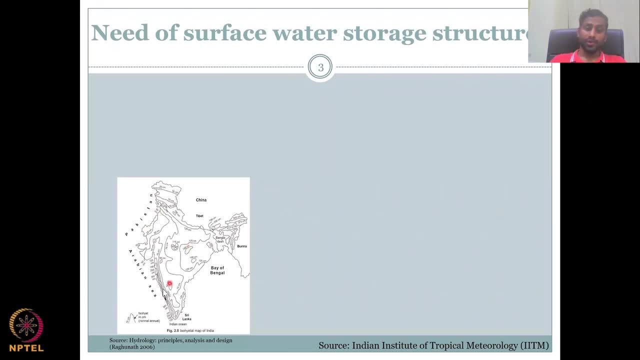 india, and even within a village or within a district, you can have a high rainfall zone and then shared with a no rainfall zone or a rainfall shadow zone. this leads to variations in rainfall and or skewness, what we call is how rainfall is less in one area and high in another area. so spatial variability is a phenomena which occurs because 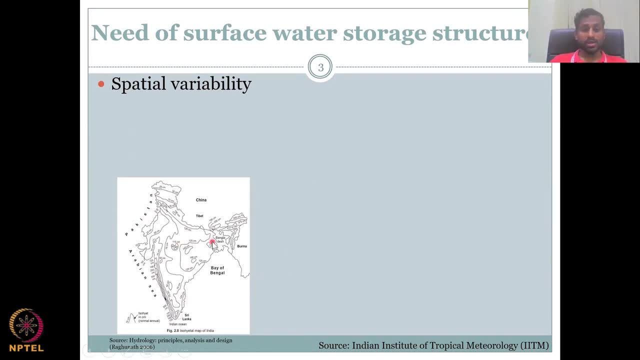 of the map you see here. it is not the same, rainfall is not the same, and if you make, furthermore, iso heights or lines of equal rainfall, you could see that there are some within a small village or within a small district. also, you will have variations in rainfall, spatial variability. 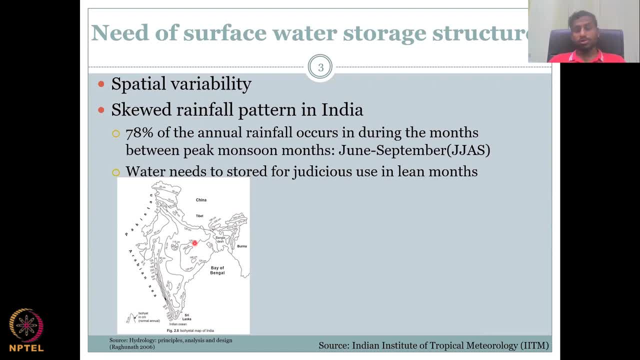 then we have a skewed rainfall pattern. what is skewed rainfall? it is not the same across every month because we are not in, for example, uh, in these regions- the northeast- you do have rainfall almost uh every single day, in the wettest part of the planet, uh, but uh, in most regions at 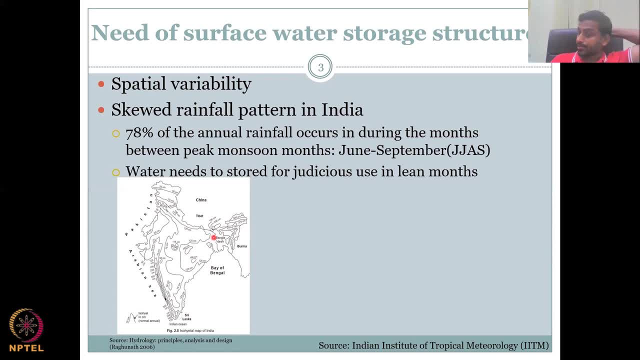 least weekly you'll have some rainfall, a very little rainfall, etc. hill stations. but most of the agriculturally active regions have a skewness which means 78 percent of the annual rainfall only happens in the monsoon months, and that too between the peak monsoon. here the peak monsoon is given as 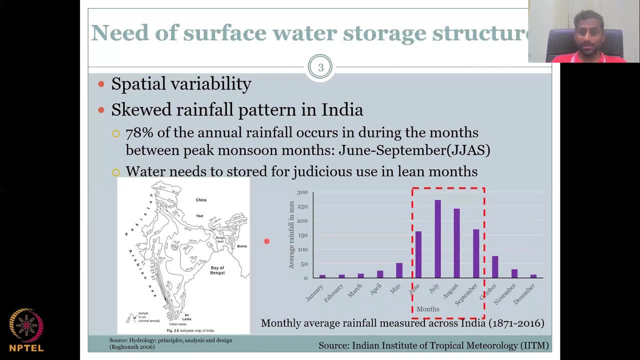 jjas, we call it, or june, july, august and september. this is kind of the overall average for india, even though it shifts. where you are, most of the uh monsoon is at the peak monsoon where the annual india's annual rainfall happens: 78 percent, almost 80 percent of the rainfall. 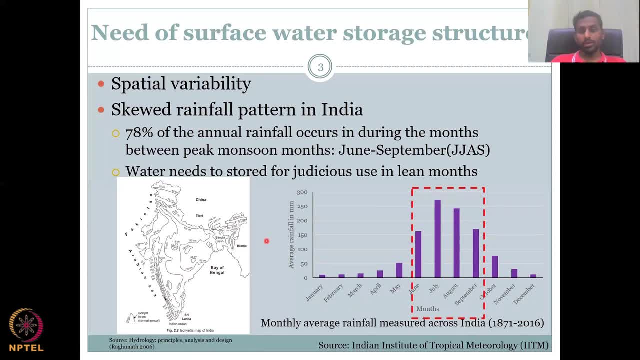 happens in jjas. if you look at it, this is the average rainfall in millimeters monthly and you have jan, feb, march- almost very uh low rainfall pattern- and then may, whereas you have june, july, july, july and may and some regions the summer extends until may, but after may you have 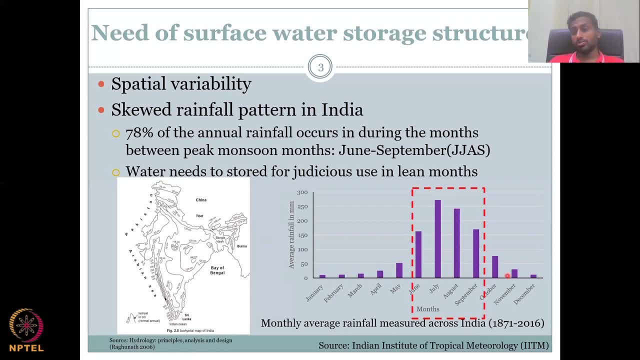 june, july, august, september. so here we say that every june 6th you will have rain in mumbai or in maharashtra. that is the onset of the monsoon. so but before we get the monsoon, the monsoon comes from kerala. so here the monsoon is coming, and while it rises here, maybe a week later after the 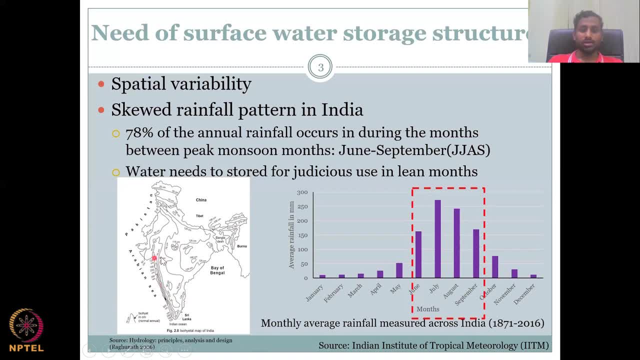 monsoon onset. we call onset is the coming in of monsoon. from there it can come here. So just a week more or less. that's why you see this variation. but it's a beautiful probable distribution, a bell curve. we call it normal distribution. 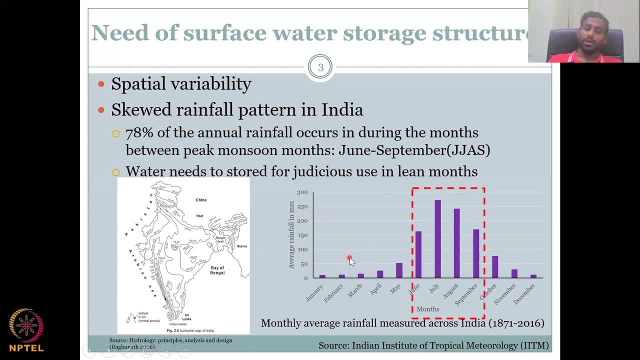 where you have more rainfall happening in a particular concentrated zone or concentrated months, which range from June, July, August and September, And then you have your winter, post-monsoon seasons rainfall. So, if you look at it, there are some regions where there's zero rainfall. 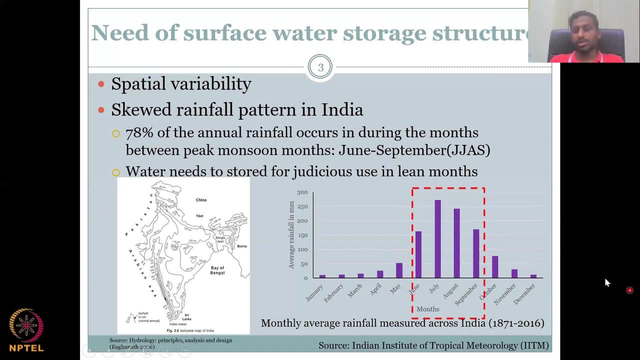 but because across India there are some regions which also get rainfall in Jan and December. We have, for example, in Kerala region. in the Northeast region you do have rainfall across. most of the time You go to hill stations, there's always rainfall right. 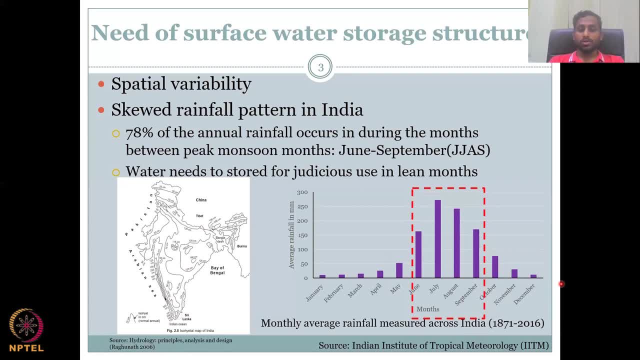 Elevation, the pre-elevation gradients, So the monthly average rainfall. this is from 1871, 2016,. so more than 100 years of rainfall from IITM Shows that this is the average pattern and there is this queness. 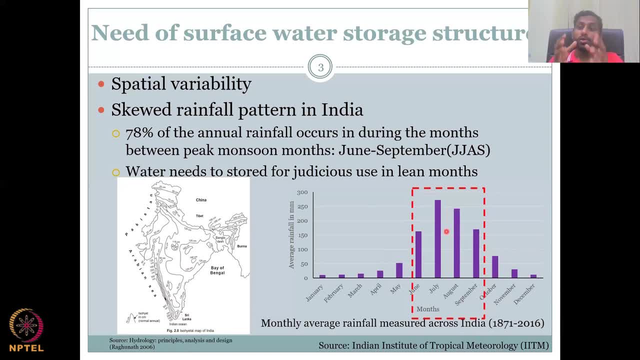 So, because it is happening only in a concentrated time, you need to capture it so that you can use it for the remaining months. What do you mean by lean months? Lean is like how I'm lean or you've have lean chicken thing. 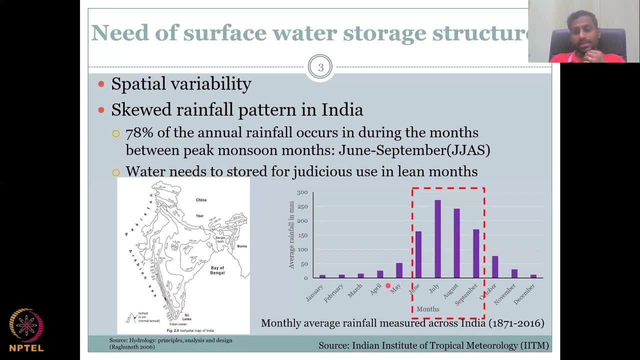 Okay. So in another word, what it means is these are the lean months, whereas less rainfall is happening. So if you say what is the average rainfall? okay, so maybe somewhere here you can draw a line Below the average, you will call lean or below average months, and then this is the above average months. 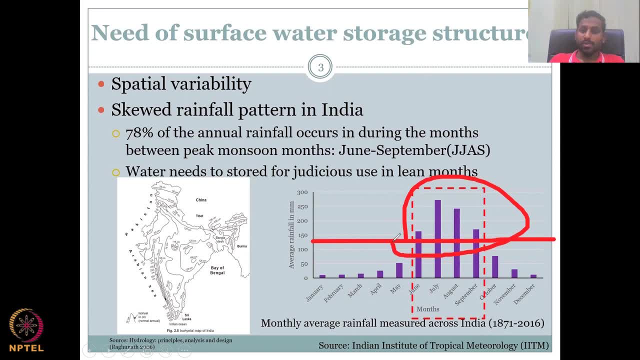 which is for sure, during the peak rainfall season you will have above average rainfall Moving on. we have to capture this rainfall so that we can use it for the lean months, both your summer spring, which is before the monsoon, and after the monsoon, which is your winter season. 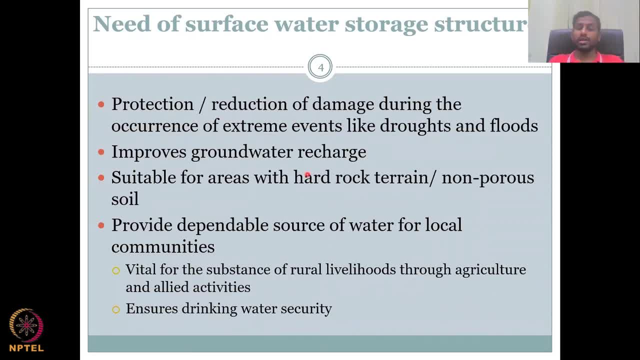 So water needs to be stored, and groundwater we saw in the previous week lecture. it can be stored but the rate is very low, So it is very slow compared to the rainfall. The rainfall can happen, For example, 50 millimeters in a week, but it cannot go that fast into the ground. 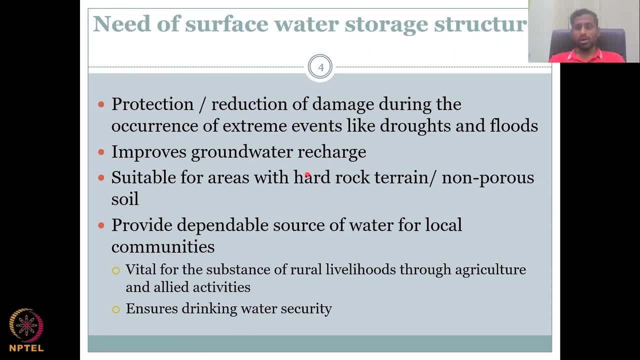 Remember it has to go infiltration percolation and then go to the groundwater aquifer. So that doesn't happen that fast. So that is why we are in need of surface water structures. It can protect and also reduce the damage during the floods and extreme events of climate change. 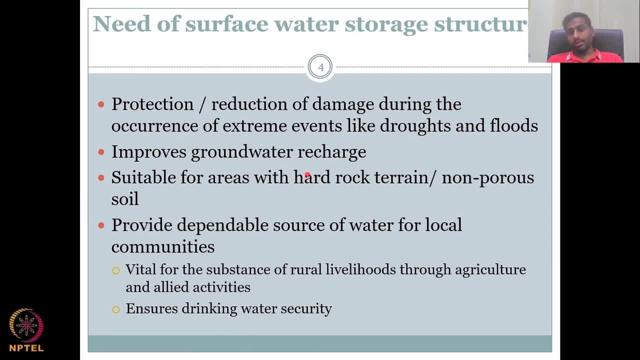 which are droughts and floods. Let's say drought. Let's take an example. You have a drought which is a less rainfall year. So if you have a less rainfall year and you've already captured the previous year's rainfall in a storage system, 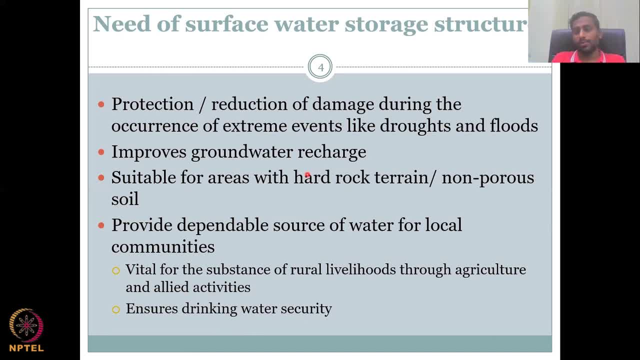 surface storage system. we will look at what are the systems in the upcoming lecture, But let's think like a tank. You're capturing the water from rainfall and river and storing it in a tank That can be used for the lean season, which is the right next to the post-monsoon season. 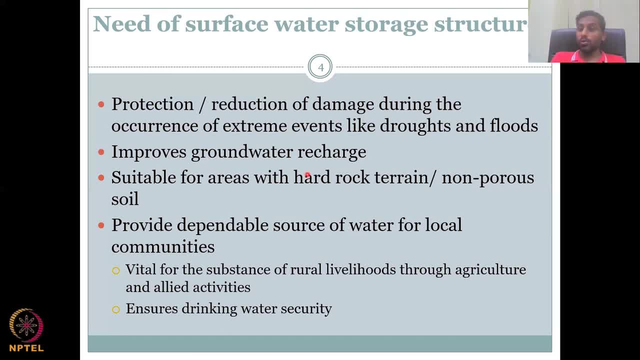 and also in a drought year. For example, 2020 was a good rainfall year and then 2021 was a drought year. If you catch the rainfall in 2020 and conserve it, you can use it in the 2021 drought year. 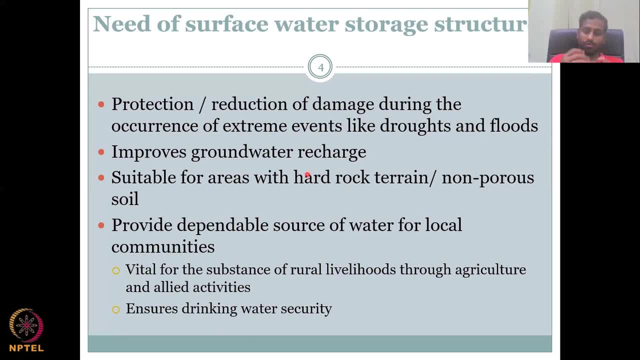 So that is what a climate extreme drought, how you can use rainfall from storage structures. How does it reduce damage in floods? Suppose you have a big flood coming through your river system and on the land and it just inundates the area. 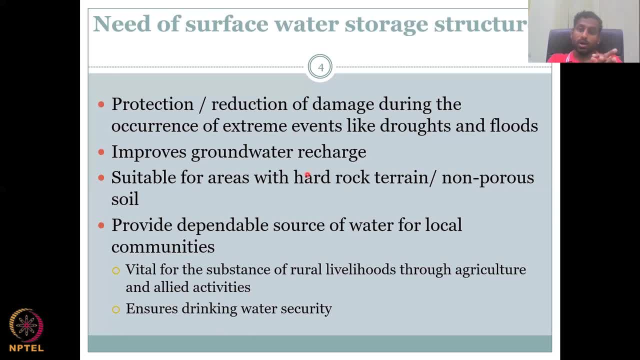 If you don't hold it, at least in smaller quantities. what happens is the water gets collected and comes downstream and floods more, So these structures actually hold this water for a particular period of time or until the volume is reached, For example, a dam. 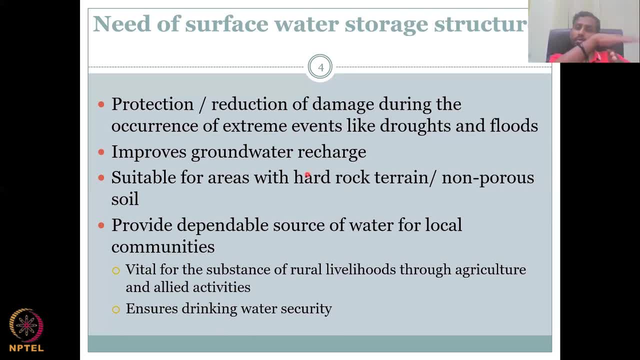 Let's say a dam, It will just stop all the water and until the dam water is full. Suppose a dam was not there and there's a big flood, All the water would come and flood the entire area. So this is how these surface storage structures help in a climate extreme. 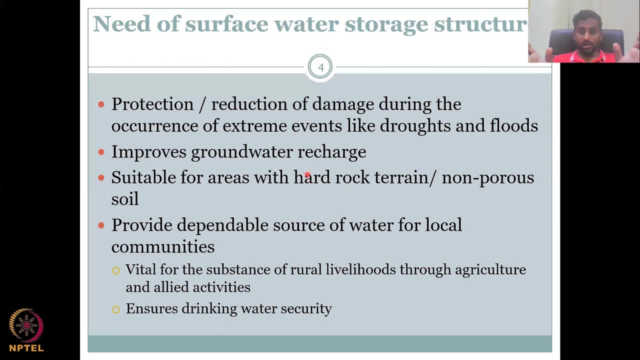 And climate extreme also means drought and flood, So in both seasons it does help. It improves low water recharge, For example, if it stores the water in the storage. the water is stored, Then there is also infiltration and evaporation is happening. 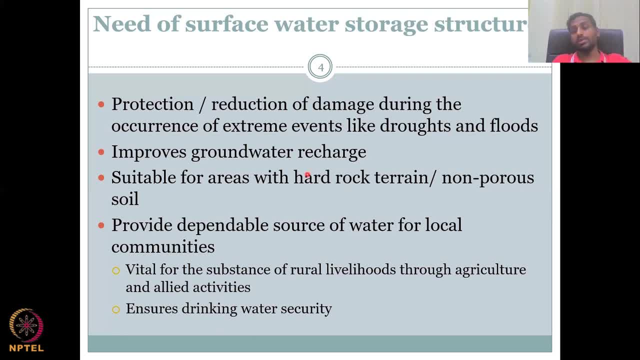 So the infiltration you cannot stop unless it is lined. Lined means you put cement on the bottom of the tank, Like, for example, a petrol tank. You don't put nothing under the tank. You have to put a lining so that petrol doesn't seep in. 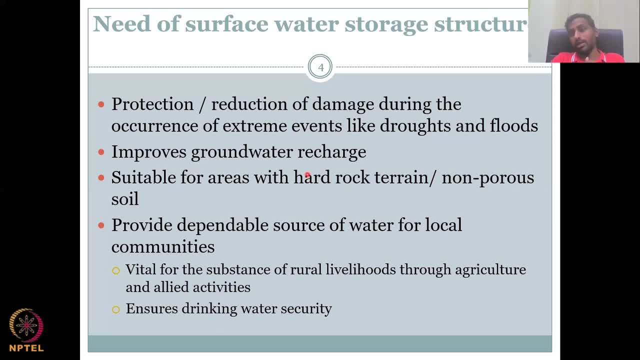 Swimming pool, You put a cement lining on the sides, Otherwise water will just get leaked into the aquifer. So we're talking about a natural system, And it's also a very important one for agriculture, where it stores the water and it can recharge. 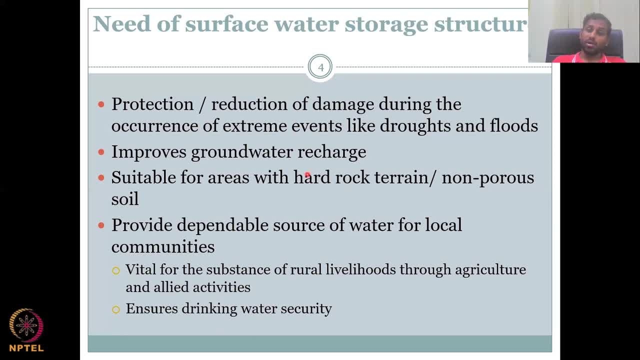 Suitable for areas with hard rock terrain, non-porous soil, because groundwater is needed and it takes a long time to recharge. So when you store this water and push it into the ground, it can recharge slowly, because you're also creating a potential head. 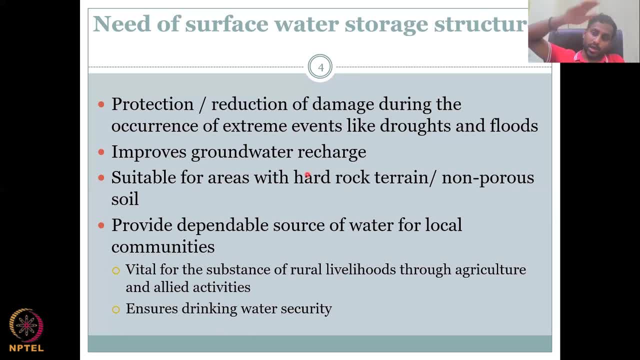 When you have a dam or a storage, the water level will rise and it creates enough energy to push the groundwater into the recharge, Provides a dependable source of water for local communities. If you look at the water storage structures like a dam or a small water lake- agricultural lake- 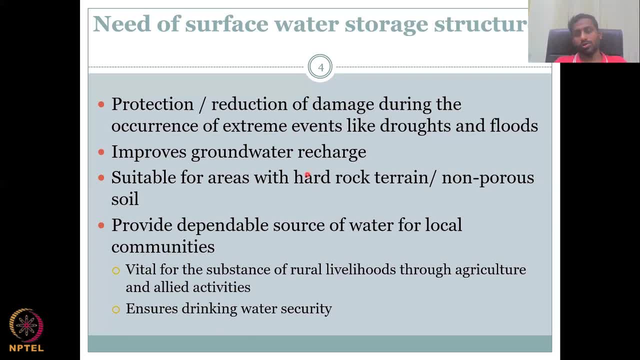 you could see that around the system, around the storage structure, there is a lively waterhood developed by the locals, For example fishing, and it could be the drinking water supply for them, And also agricultural means. So it is vital for the substance of rural livelihoods. 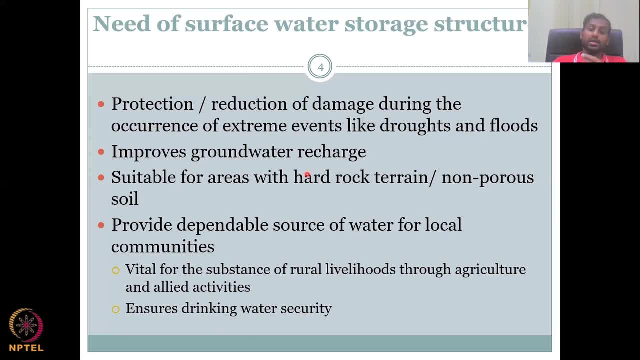 through agriculture and allied activities. When I say allied activities, it includes fish, livestock cattle, poultry, anything that supports your agricultural livelihoods, And it also ensures drinking water security, even though drinking water is less compared to the use of other units. 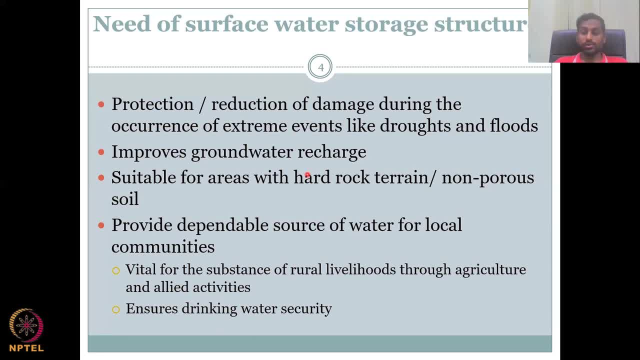 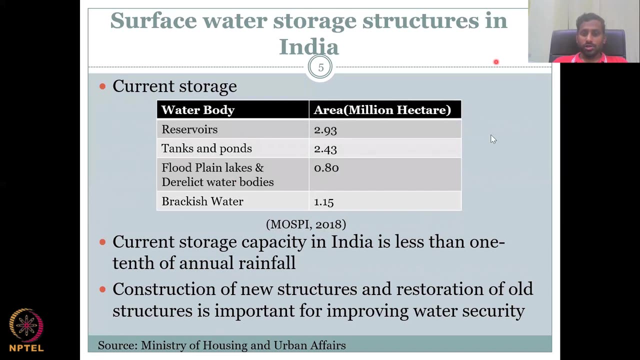 that I've described. Still, it is vital for the substance of rural livelihoods and it is very, very important. So these structures could provide good drinking water source during the lean season, which is drought, or the high flood season. Let's take a look at the surface water storage structures in India. 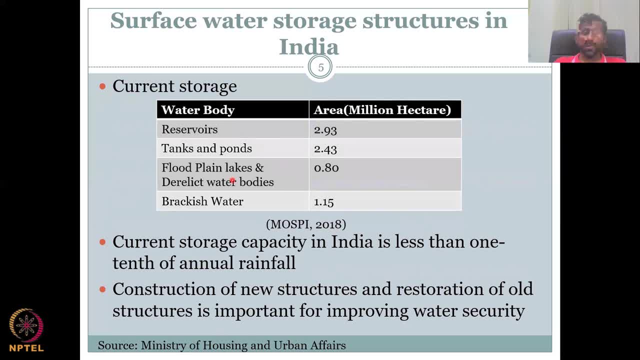 So the current storage, as per MOSPE 2018, says that the reservoir is around 2.93 million hectares. Tanks and ponds occupy 2.43 million hectares. Floodplain lakes and derelict water bodies are around 0.8 million hectares. 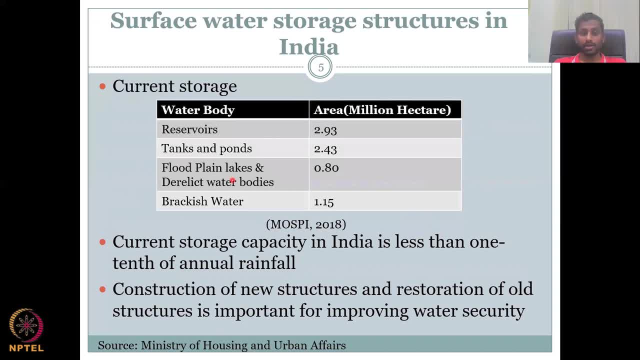 And brackish water is 1.15 million hectares, So this gives a good understanding that your reservoirs, which is tanks and big storage structures, occupy the most area in India, followed by tanks and ponds. The floodplain and brackish are smaller. 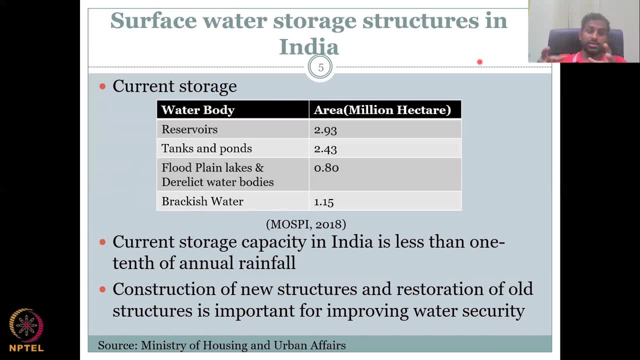 However, your tanks and ponds- small tanks in villages and small tanks in villages- and your rural ponds still occupy a good chunk of space. The current storage capacity in India is less than one-tenth of the annual rainfall. So if you compare this volume, so this million hectares. 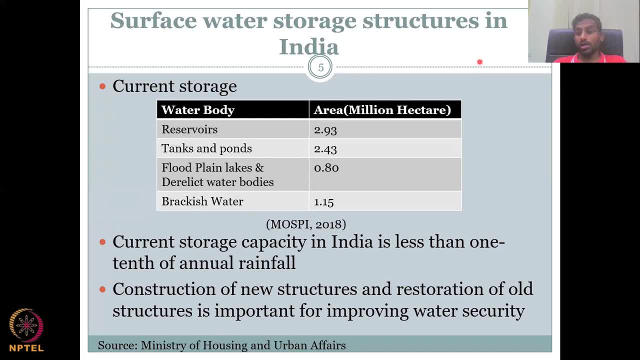 multiply the thickness and the total volume stored and then you compare it with the volume of rainfall we have. it is not even one-tenth of the annual rainfall, which means 90% of the rainfall is let to go into rivers, water storage in groundwater and etc. 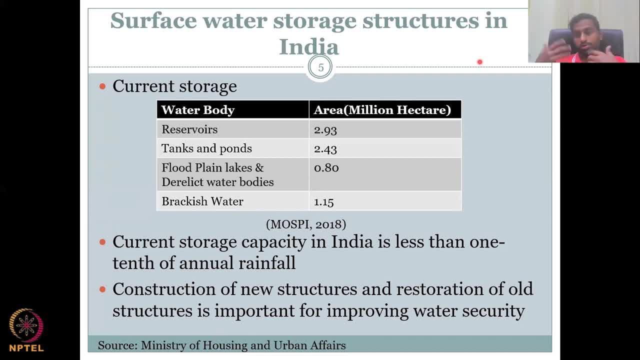 Is it good or not? That is a different question, because you still need your rivers and lakes and streams to flow. But is it all washed away into the oceans and seas is the question. So that number we don't have exactly. we need to calculate. 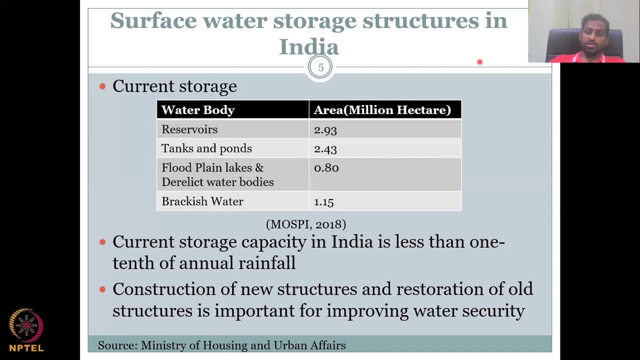 So construction of new structures and restoration of old structures is very important, because we are losing a lot of water into the oceans and rivers, which can be captured. for a water-hungry nation like India, where agriculture is predominantly using a lot of water, 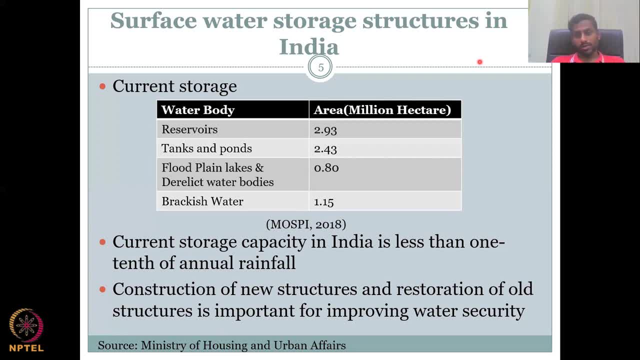 and it is very, very needed to have this water supply. Not only India, but almost all South Asian countries are water-hungry, which means the population is increasing. There is a demand for water: water to sustain the livelihoods and demand for agricultural productivity. 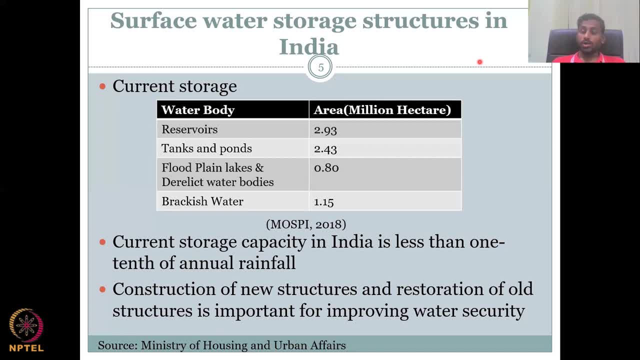 So all these countries are actually wanting more water. You cannot create water, So you need to store and then capture as much as water is there And, given the transboundary natures and international, you know issues in getting the water between countries. 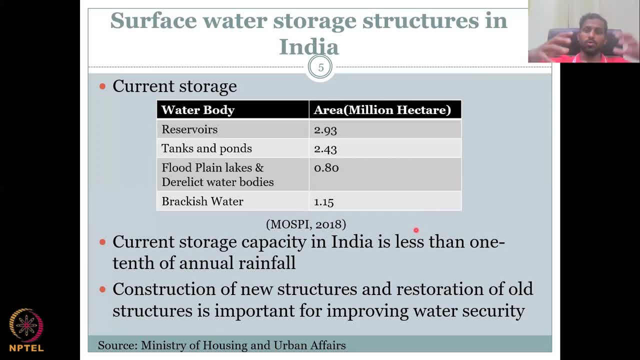 it is always smart to at least use the water that you collect in rainfall. So capture it, use it and then make sure you're not wasting too much water into the oceans and seas, considering your agricultural needs. So let's continue looking at the large dams. 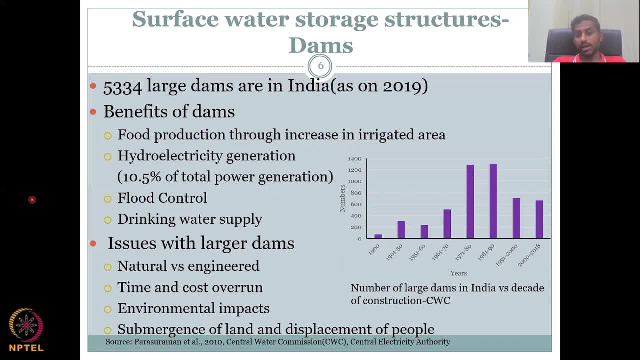 So it is, 5,334 large dams are in India as on 2019.. And these large dams is one type of a surface water storage and it is the biggest. Okay, So this is what our dam looks like. We love some images, but dams have their own positives. 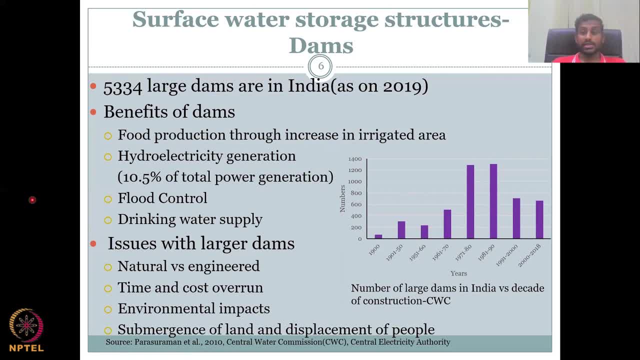 which are the benefits of dams include flood production, because it is a massive storage. It is a couple of feet high. you know, like it's not, like you cannot just jump in and swim for days, you know it's too big. 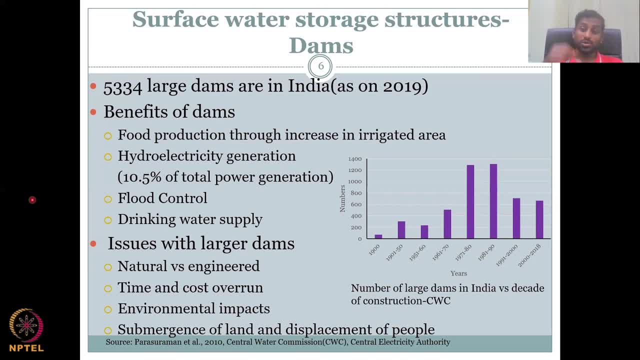 So dams are pretty pretty. that's why you cannot allow- you're not allowed- to swim in a dam zone. It's massive, So it can actually capture the flood water and buffer act as a buffer, which means a storage space where excess water can be put. 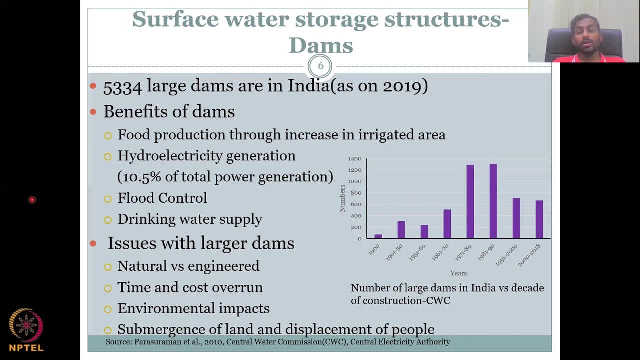 Okay, And it also increases your food production because you have an irrigated area. So once you store the water, that water is released into the command area we call wherein water goes into the land, for agriculture is supplied in the. 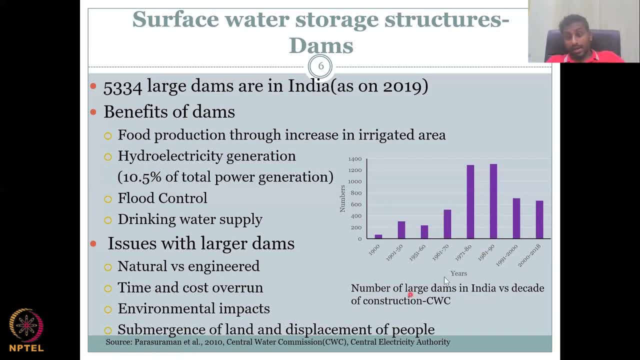 in the land for agriculture. If you look at the number of large dams, so there is a difference between large dams, check dams, and small dams, medium dams. So large dams are the biggest, which are not only for irrigation but also for hydroelectric generation. 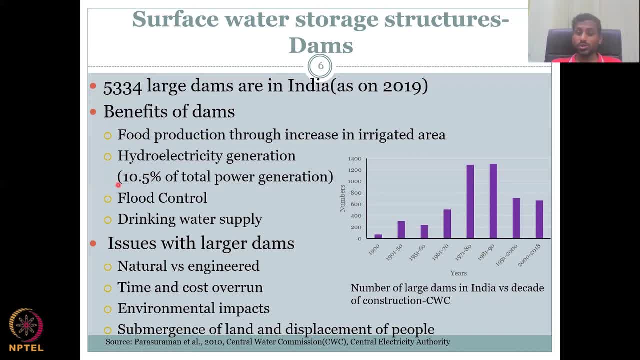 which accounts to almost 11%, 10.5% of total power generation. So also India is in need of power- right electricity- because we are also pushing industrial development and we need a lot of power. We have solar and et cetera. 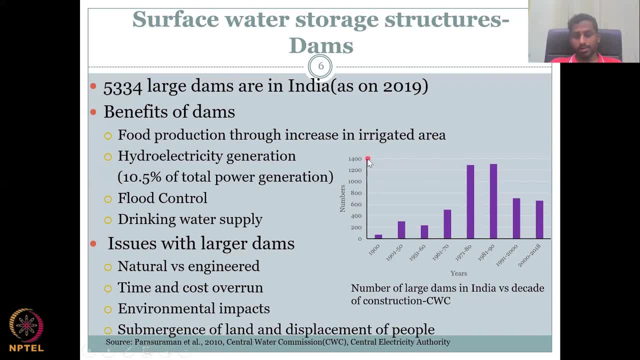 But hydroelectricity is also generated. So if you look at this, you have the number of dams, big dams, large dams in India, And it's not easy to make these dams right because before the British gave us independence, when they were ruling us. 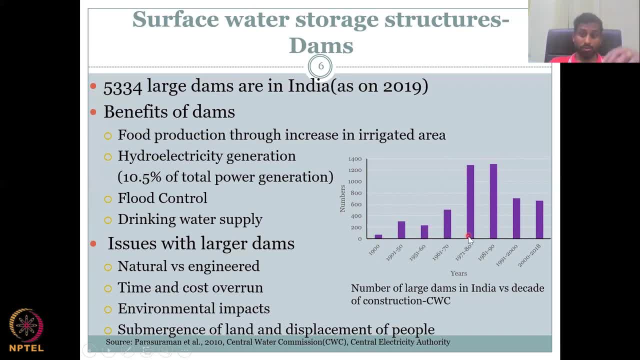 So you could see that not, they built a big, big dams and still operational, but it was slightly managed. Their motives were different. They didn't want much for India, They didn't want much for India's development. But after India's independence, that's when we started to push more on the large dam scenario. 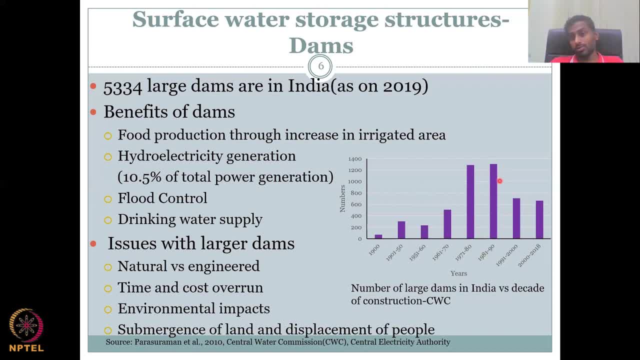 And then because of the anti-benefits also, or the issues with large dams, there has been a slowdown and not much you can build. Also, the lands are already occupied by large dams. So let's look at some of the positives. 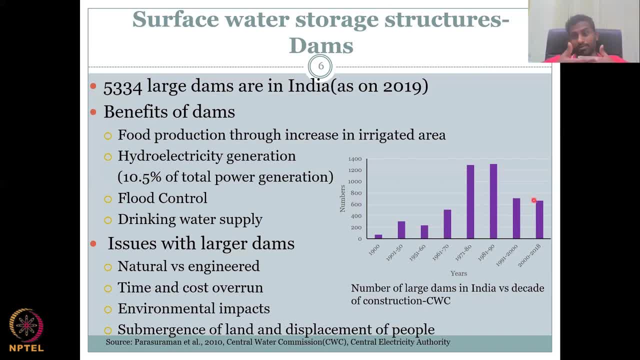 As I said, food production is increased, Hydroelectricity is increased Flood control. it can buffer the flood water And all this water can be piped into a water supply. For example, all the dams in Pune areas are catering to the drinking water supply of Mumbai. 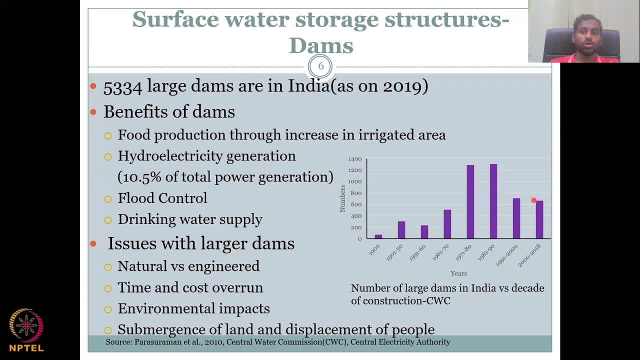 Because in a city of Mumbai you cannot afford to put a dam, It's too expensive- the land where it is the industrial capital of the country. So where would you, sorry, the economic capital of the country, where would you put all these, you know, dams? 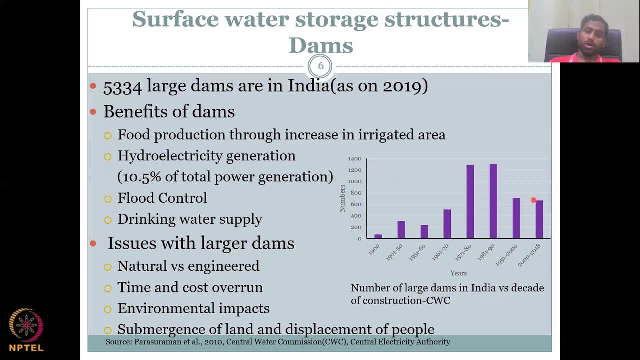 You cannot, So the water supply is taken from outside. Similar in Delhi. you know water is taken from outside, So these dams do help in drinking water supply, not only for that region but for miles and kilometers away. But there are a lot of issues. 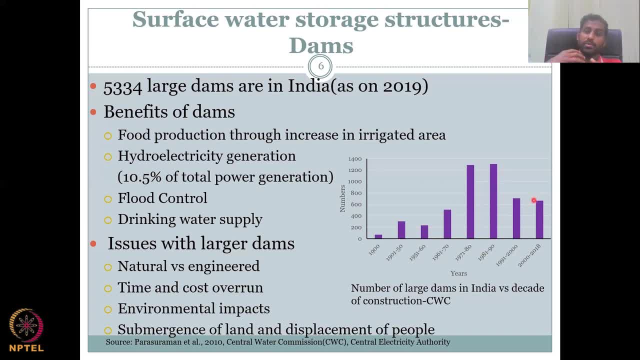 If you look at dams, there is a difference between naturally managed water and engineered. Dams are more engineered structures, which means it is kind of there to stop the natural movement And it's not. it's not accounting for the natural dependencies of water. 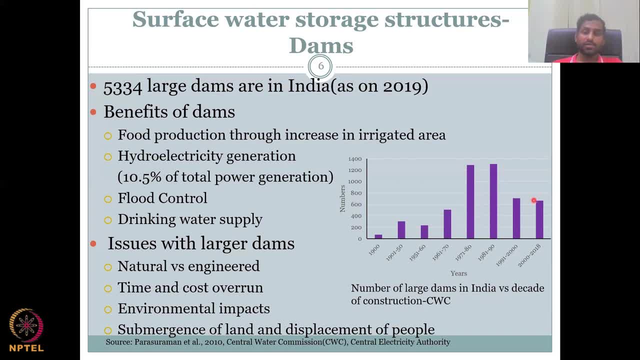 For example, you have downstream, you have e-flow, which is the environment requirement of water. So all this is not thoroughly taken up by large dams. There are some issues: Time and cost. overall there's a huge cost involved and time to build it. 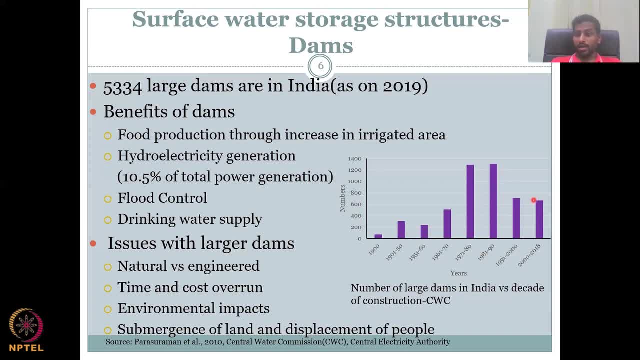 Just recently you would have noticed the Uttarakhand dam. they built it in such large time and money but it just got washed away. There are a lot of environmental impacts. You have to clear the land. There is a lot of people's livelihood. 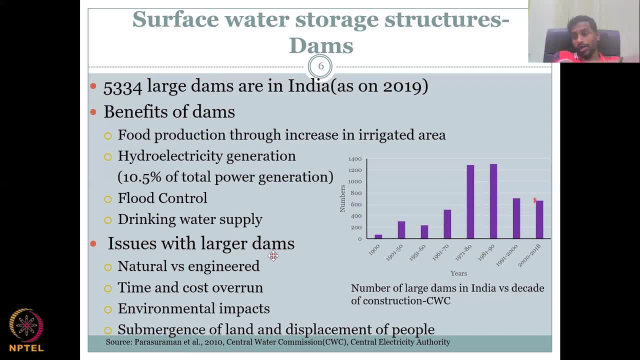 Displacement happens. You have to clear the land, take the people away, relocate them. All this happens because it's a huge area. When you stop the water, a huge area has to be flooded And that becomes the flood, becomes your dam water correct. 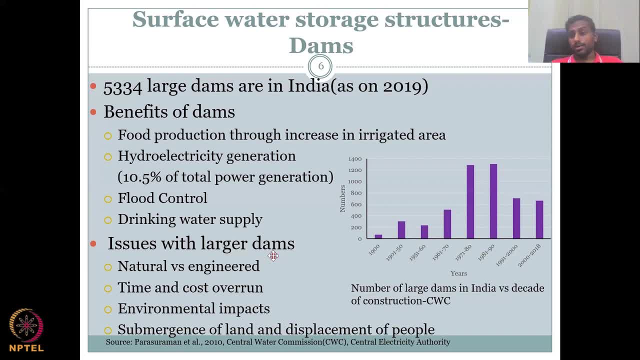 You just stop the water. One more thing is the size. not only the size alone, But also the environment factors. as I said, it has to cater to the movement of water, So some environmental benefits are lost if you stop running water. 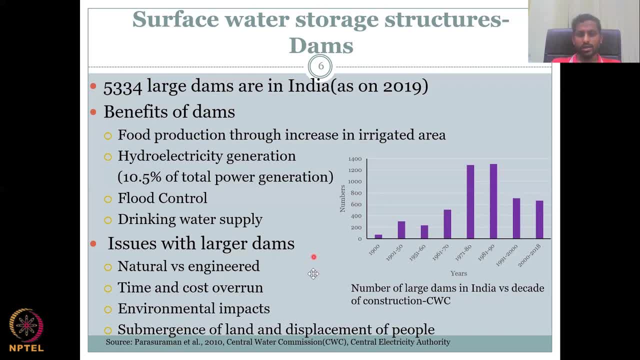 Okay. so these are mostly noted as the negatives of, or issues of large dams by these authors given below. So you could see that, as I said, most of the dams were did only after the independence. but there is a question: how did our ancestors do this? 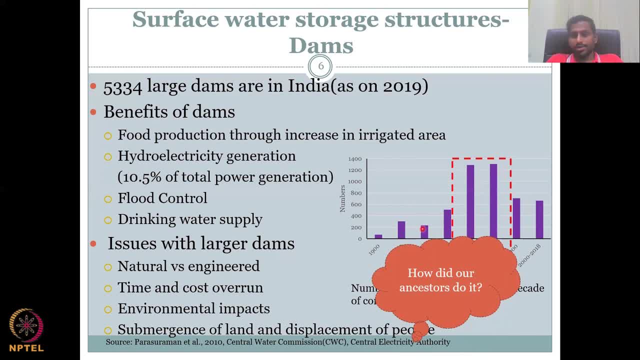 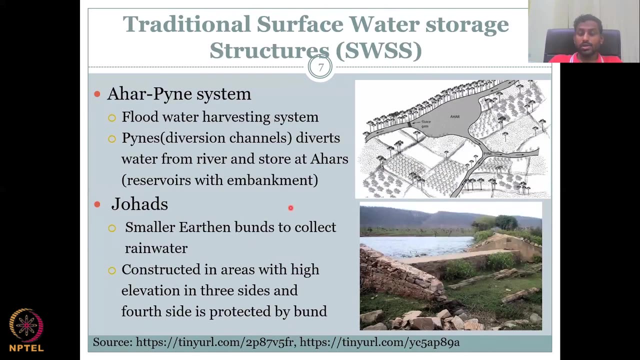 If we know that dams were less during the British era and before that it was really really less 1900s. So how did our ancestors, kings and others who ruled before the Britishers, how did they control this water? 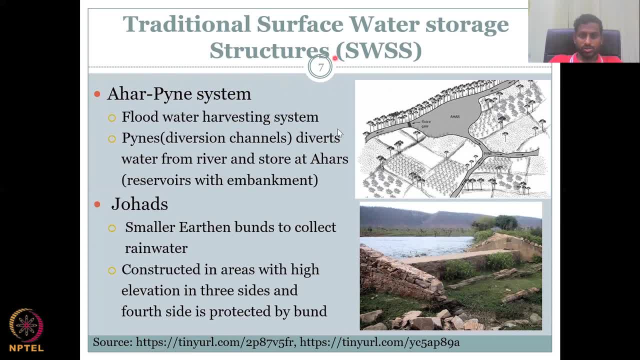 So there is a lot of traditional water resources storages. We call it surface water storage structures as SWSS. So this is just in short, to put it in the slides. So there is multiple methods: There is traditional, there is nature-based methods and there is engineered methods. 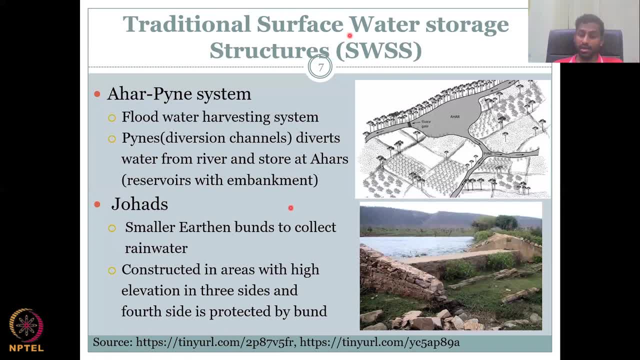 Let's look at the traditional methods to understand how their ancestors did it. So the first one we would look at is the Ajaar pine system, where flood water harvested through a small area demarcated in the villages and pines are the diversion channels which 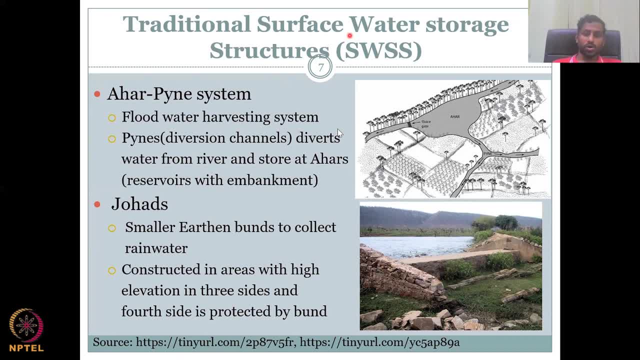 take the water into these small stores or storage regions as Ajaars, which is reservoirs with embankment. So it's a small reservoir, kind of a small dam, but it is made with embankments. not much cement used, not much land is cleared. 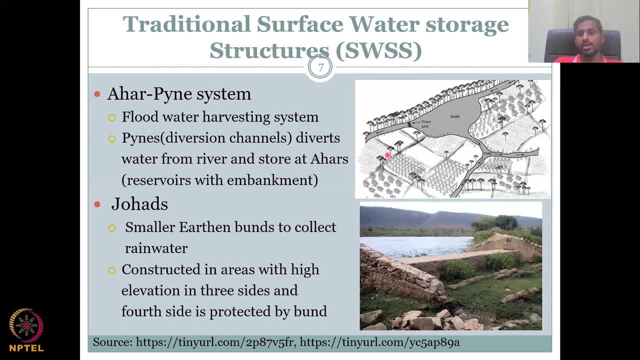 So normally what the traditional ancestors did is to find a low-lying area in the village, and in that low-lying area already water would have been stored. So all they had to do is clear the land, put embankments on the sides and then channelize the water. 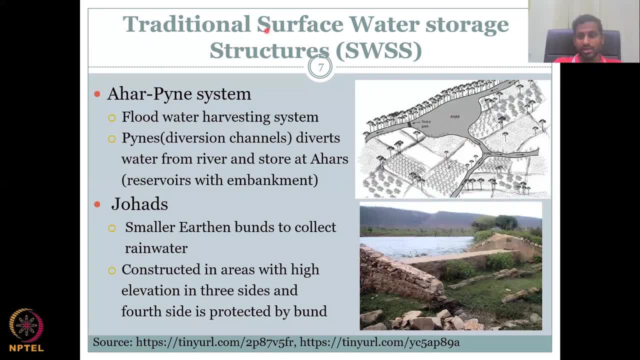 So, instead of water moving in every direction, like, for example, like this moving in every direction into the Ajaar, they would just make sure that it is all pooled into one channel. So this is how they managed this important capture: the rainwater. 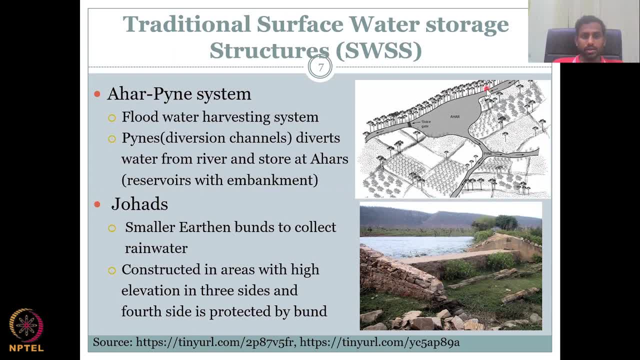 So they just channelized it through these pines, which are diversion channels, and into Ajaars, And then they might have some blocks to stop the water, for example like this, And from that blocks after a particular height is reached. people can use it for fish, drinking livestock. 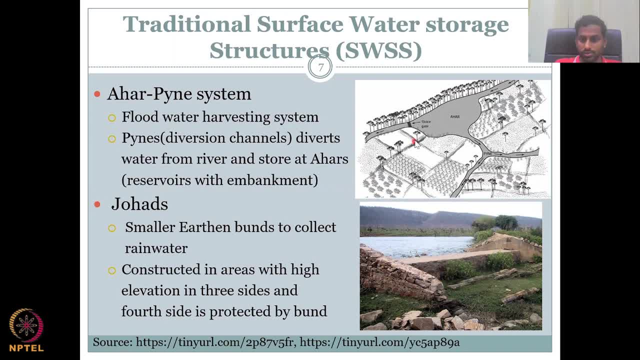 and also put smaller channels, like this loose gate, and then take the water into the villages, into rural lands, For example for agriculture. Johargs is another similar type where smaller earthen bunds to collect rainwater are done. It's not as big as the Ajaar pine and it's constructed in areas with high elevation in three sides and fourth side is protected by bund. 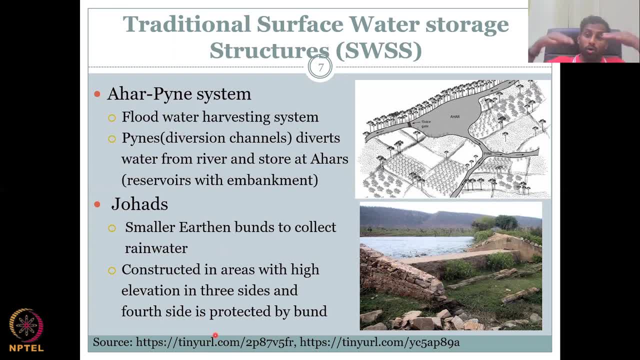 So, for example, you don't have a low-lying area in the village. what would you do? So all you do like, for example, here all is elevation land. you would pick an area where all these four elevations are high and the smallest elevation, which is the smallest height, land is used as a storage. 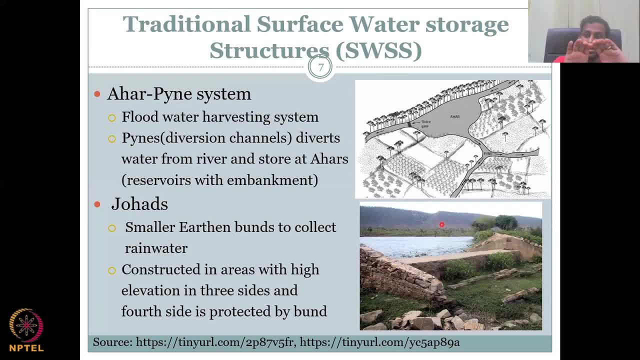 So you just build a small earthen bund. A earthen bund is a structure like this and earth is just mud, sand and stones. It's not concrete, which means earthen bunds still can do some recharge, still can have some leakages, which are good. 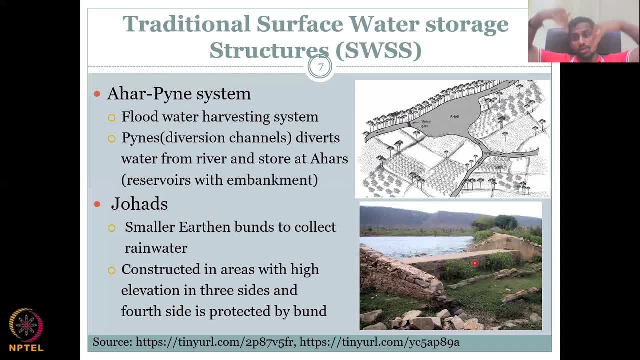 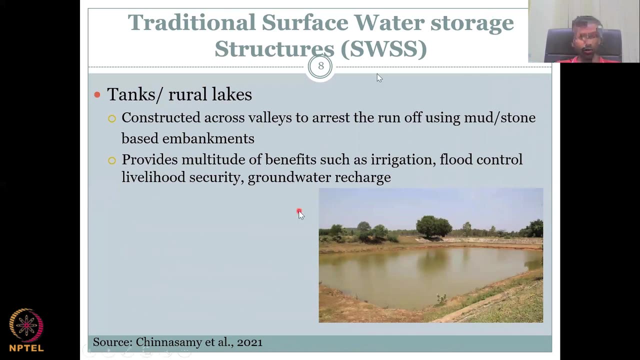 And so this bund actually stops the water from these high elevations and starts a pool, So that pool of water can be used as a surface water storage. Moving on, we also have another very important structure, which is tanks in rural lakes. 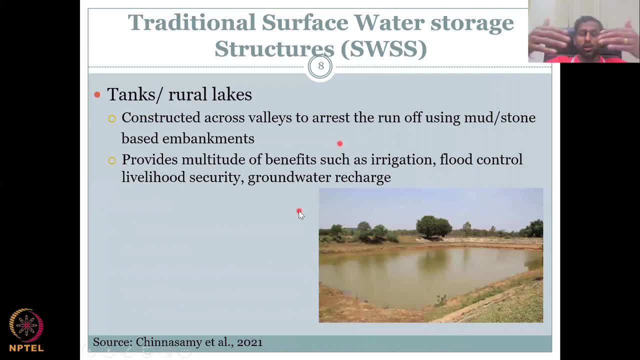 So these are demarcated, simple land which is channelizing water into and storing the water. So it's constructed across valleys to arrest the runoff. So small, small valleys you will have and all the runoff is arrested. 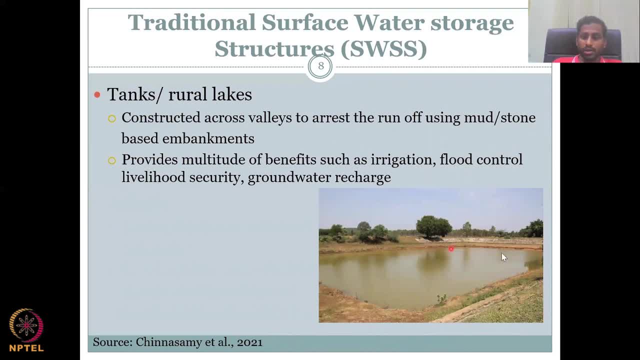 And put into it And around the area you will have mud or stone-based embankments. So basically, the ancestors just dug this area through hand and plows and stuff made a deeper thickness of like a bigger well And then all this water would come in and on the surrounding edges they made these embankments. 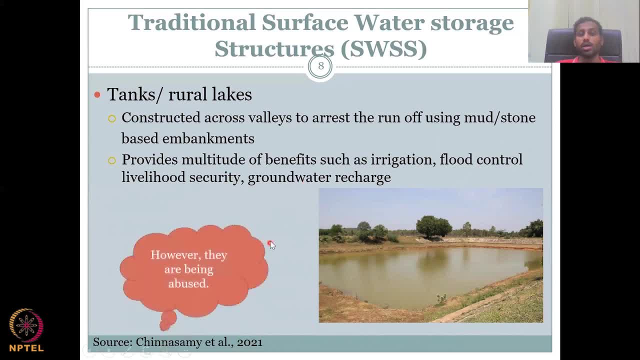 Provides multitude of benefits, such as irrigation, flood control, livelihood security. groundwater recharge. So because this is mud, This is not lime, which means no cement is at the bottom. Groundwater does recharge, Excuse me. So therefore it provides multiple, multiple benefits, not only for irrigation, not only for agricultural water use. 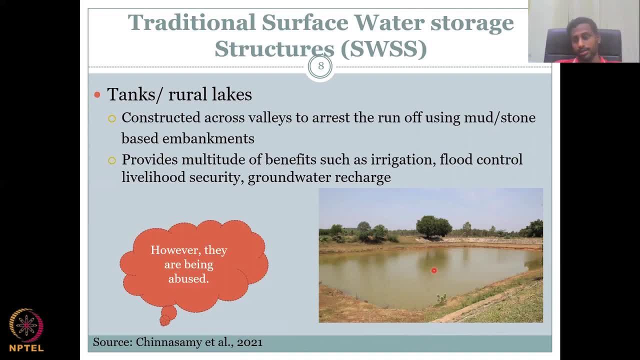 Flood control, as we saw, livelihood for fish and then for food security, et cetera. And sanitation- people used to bathe there- and, most importantly, groundwater recharge. How are they being abused? They're not protected well. 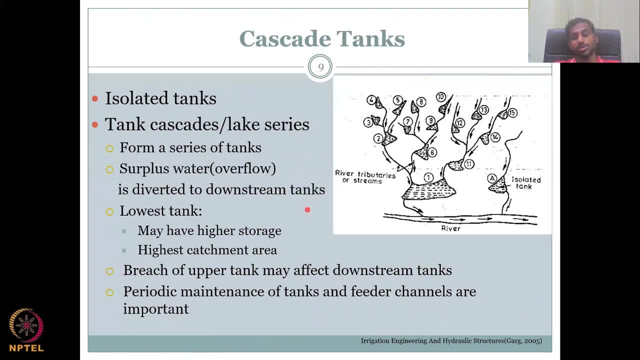 If you look at it, we will cover some issues of these tanks in the next class, But you would notice that in the villages these tanks are not protected properly. As long as the tanks, we also have another tank system called the cascade tank system. 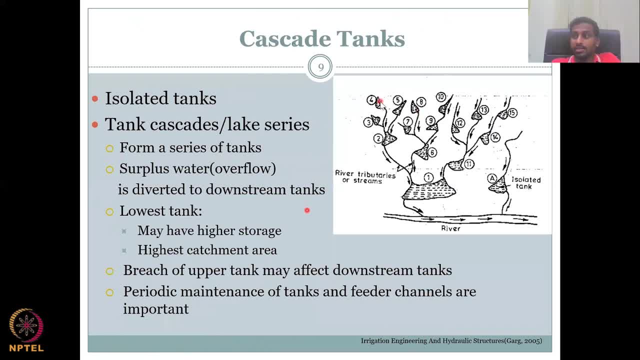 So just visualize we had one tank. So this is just one tank in the village. So this is just one tank in the village. Think about placing small tanks and connecting those tanks. So the ancestors are very smart. They thought, okay, first let's make one tank. 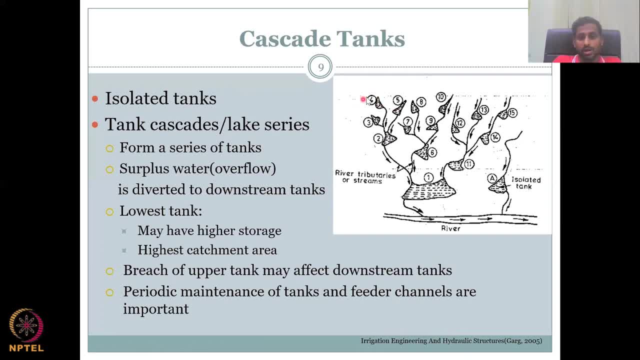 And this tank could cater to the hamlets or the houses and villages around this tank, But then it can. water can still go to another tank. So as one tank fills up, it goes through the channel and then fills another tank. So only after number four fills up, number three fills up and then number two fills up and then the bigger tank, number one, fills up. 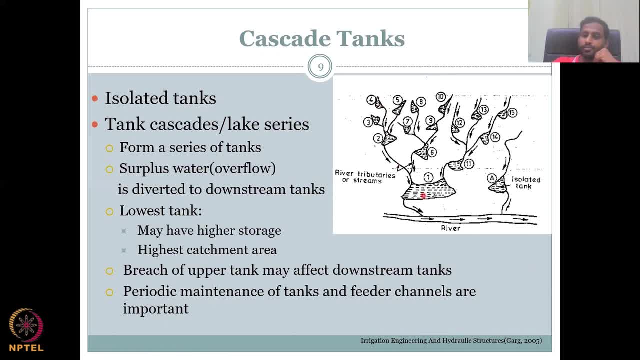 And they built it along the tributaries also, which is this line, you see. So the river is like kind of stopped and a big tank is made. It's not a check dam, it is a big tank. So water flows into the river and when water flows, a big tank is first filled up. 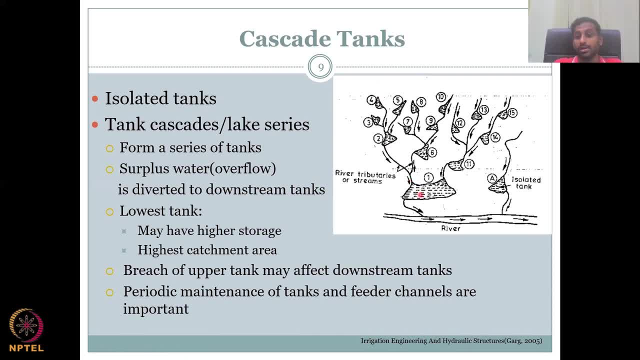 And after the tank is filled up, the next tank and the next tank until the bigger tank is done. And once the bigger tank is full, it goes into the massive river, out into the system. So all these are very, very important. 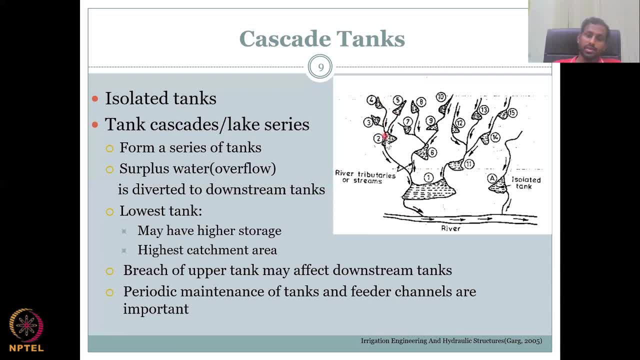 And these are called cascading tanks. So one tank is filled and then another tank is filled, another tank. What we saw in the previous slide was an isolated tank. You just had a channel and then the water was filling. So what is the benefits of tank cascades? 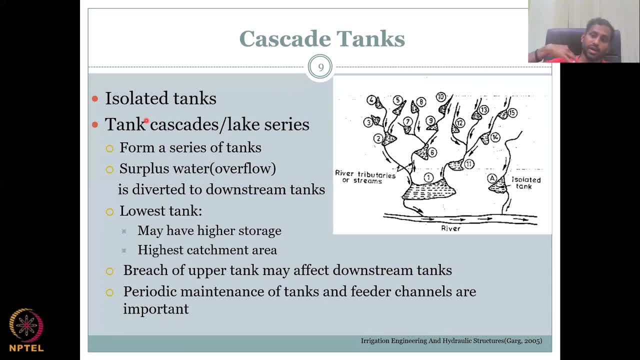 It is a series of tanks, it's not one tank. So when you manage, you have to manage all the tanks together to get good water in number one, Okay, And then there is always surplus water is being taken from one tank to the other tank through downstream links. 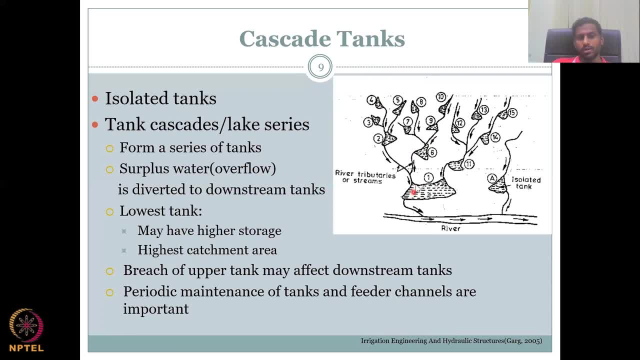 Okay, So these are the downstream links where water would come. The lowest tank may have higher storage, which is the lowest rank, or the lower elevation tanks has more storage because it can take the water from multiple resources and has the highest catchment area. 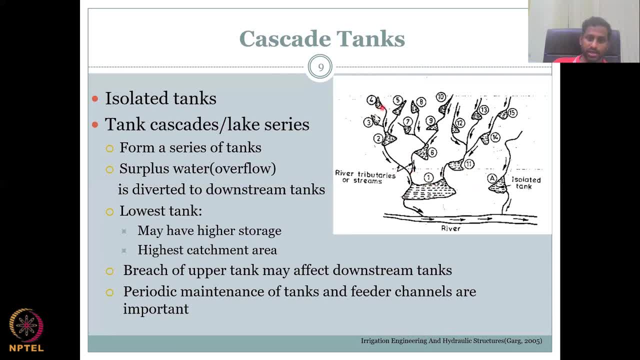 So this catchment area is the highest compared to this tank, which is: this is the catchment area. The breach of upper tank may affect downstream tanks, So that is why it is very important to manage And, as I said in the previous slide, most of these tanks are not well managed because 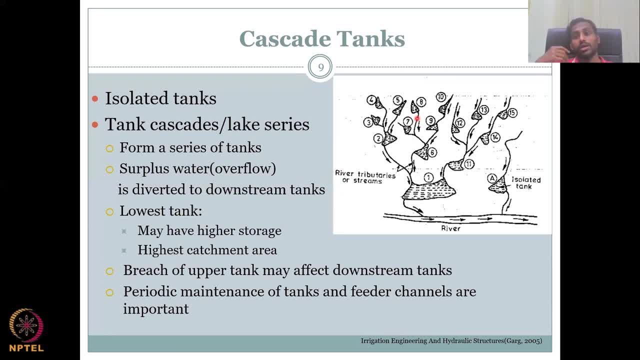 we'll look at the reasons in the future class in this week. There is no community participation, There's no funds for it, People don't take ownership, So all these issues are there. So there is a breach of upper tank and if that happens, mostly all these tanks won't work well. 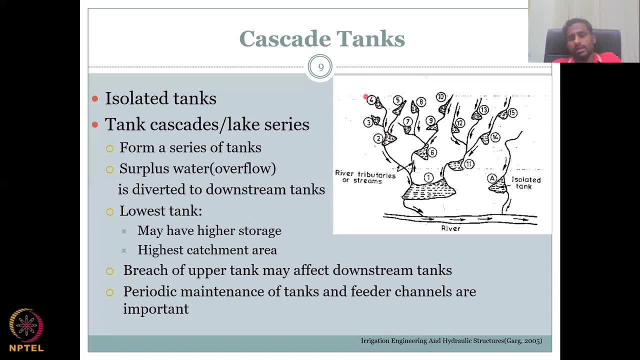 because all this water would come down and then we lose this land and then slowly this tank will also get broken because of this water coming in and slowly all these tanks will erode. So after one tank breaks, all these tanks, other tanks slowly will break. 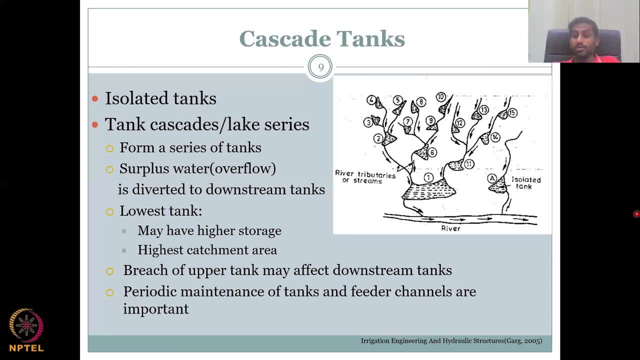 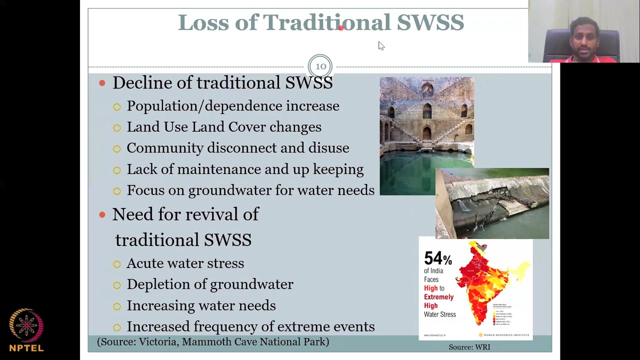 Periodic maintenance of tanks and feeder channels are very important, and even the trans boundary tanks and trans boundary connecting channels, like the one in Koshi, have to be properly managed and periodically maintained, Otherwise a lot of issues can happen. So there is a loss, a lot of loss of these tank systems, of traditional tank systems. 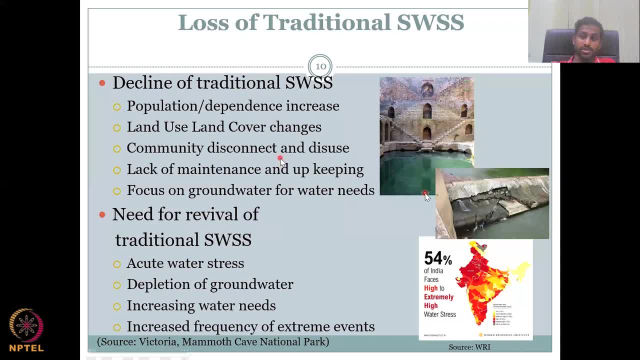 Let's see some of the reasons, and we'll also touch upon this in the upcoming lectures. There is a decline of traditional systems, surface water storage systems, especially because of population and dependence increase. When population increases, people start to abuse and they take more than they want, because 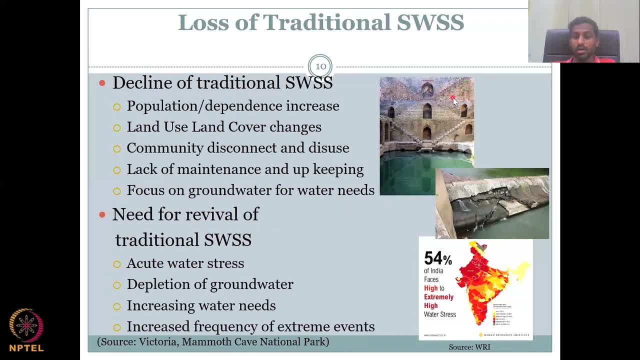 of fear of others. would take it, For example, here. if you could see water was around here, but then not proper maintenance. You can see trees growing, the rocks broken, the stairs broken, all of it. So if you don't manage it, and people are using it and so they should also manage it. 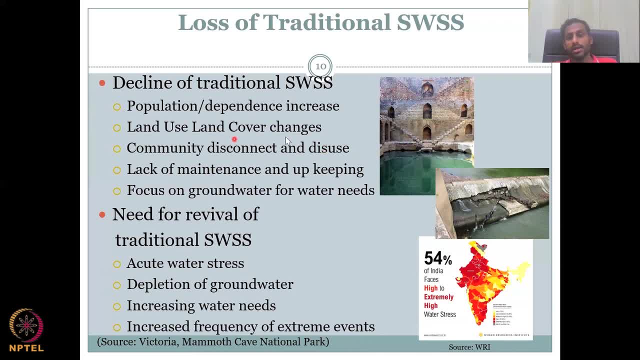 either the government or the local people. Land use, land cover changes because you tend to abuse it, you tend to encroach it. these tank systems are gone, the traditional systems are gone, coming to disconnect and disuse. as I said, If those who are using are not going to take care of it, we will lose the tanks. 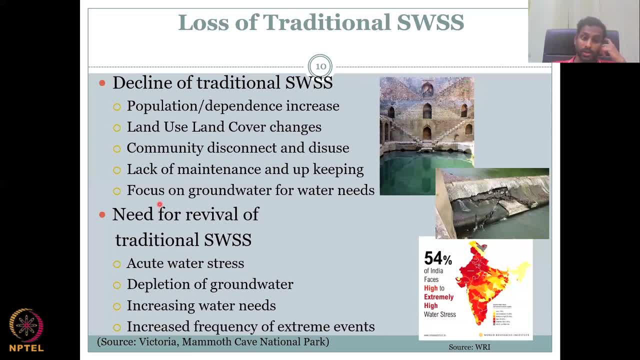 We will lose the water bodies, the ponds, Lack of maintenance and upkeeping, There's no ownership, there's no money set for these revival of these systems and people don't understand the connection with groundwater. and also people have the access to individual groundwater, so they have just started to abuse these systems. 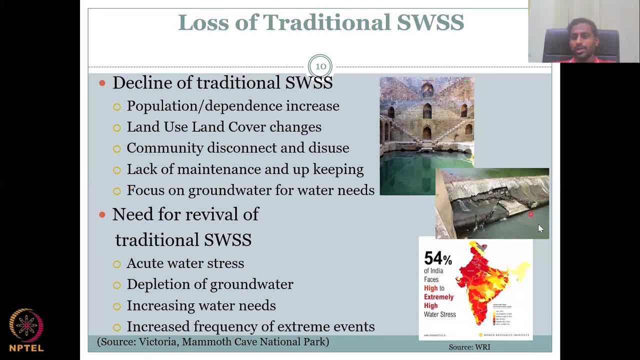 They don't care about. look how it's broken. and once it's broken, slowly it gets demolished and no one takes care of it. So there is a need for revival of traditional SWSS, especially because India has already 54% stress and it is going to increase pretty bad, as per this report. 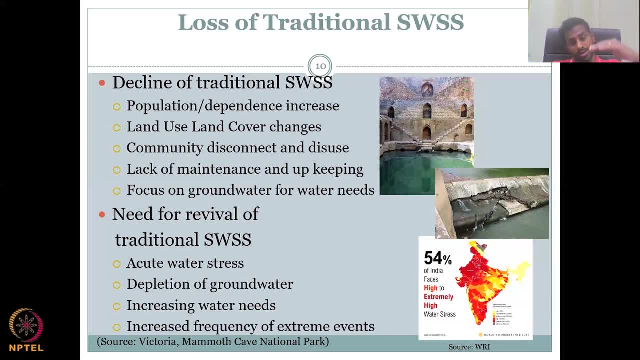 Acute water stress is going to happen. Groundwater is already depleting And the increasing water trends, as I said, because of population and overuse, Lifestyle has changed. Everyone wants to wash their car using fresh water. you know which is not correct.